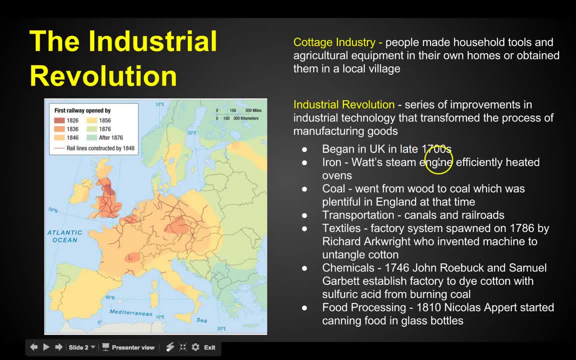 In fact, in the late 1700s, here when the Industrial Revolution begins, you have iron, Something that takes a long time to heat the ovens consistently with wood, But with the invention of Watt's steam engine it efficiently and cheaply heats ovens over an extended period of time. 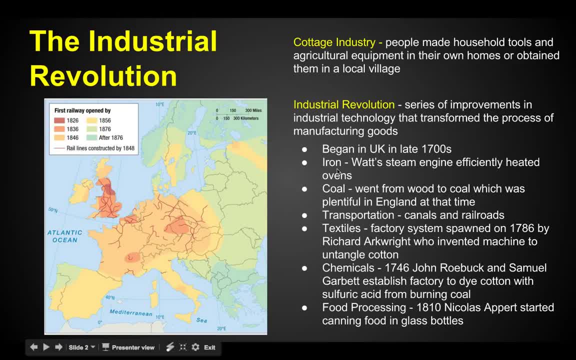 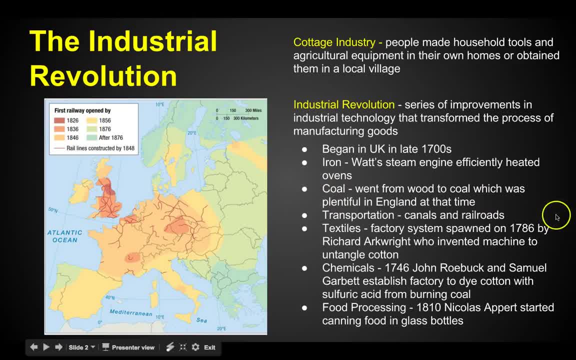 So again we went from wood to coal, and that was something else that helped Europe explode in England as far as the Industrial Revolution. So again we went from wood to coal, and that was something else that helped Europe explode in England as far as the Industrial Revolution. 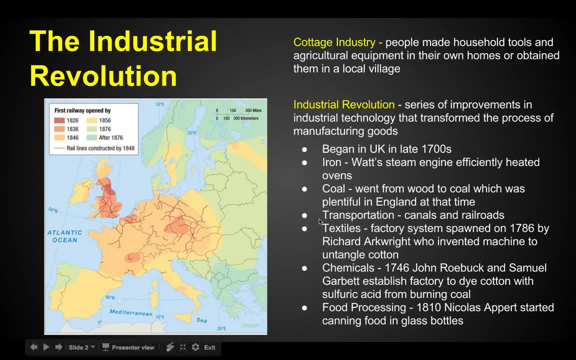 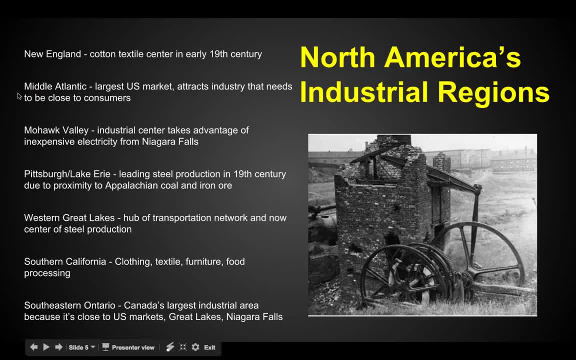 Textiles, clothing. this factory system was spawned on in 1786 by Richard Arkwright, who invented the machine to untangle cotton and millions of people. it's going to be the largest market you can sell your goods to people. there's tons of people there, mohawk valley. it's the industrial center it takes advantage of. 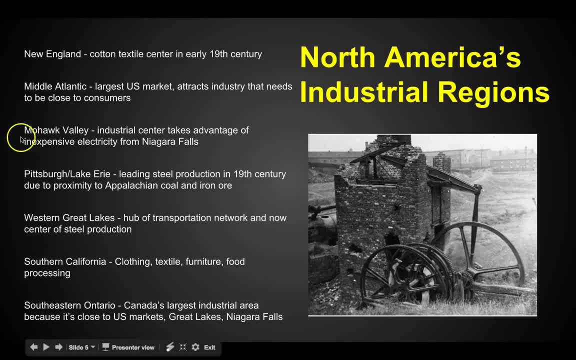 inexpensive electricity. from niagara falls a bunch of water flowing, you can make electricity very cheaply and efficiently. pittsburgh lake erie it's leading steel production in the 19th century due to its proximity to the appalachian coal and iron ore in the mountains there. 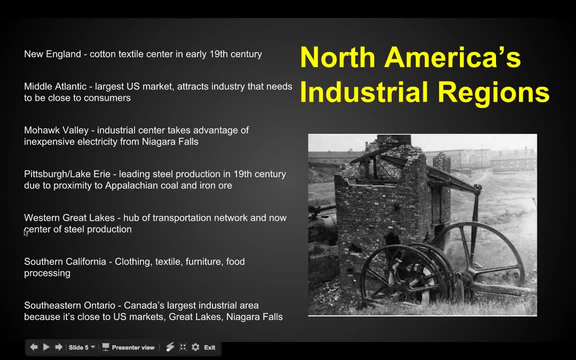 but the steel moved on westward to the western great leap, to the western great lakes. it's the hub of the transportation network and it's now the center of steel production. you think about trains and airplanes out of chicago o'hare international airport, all the cattle being. 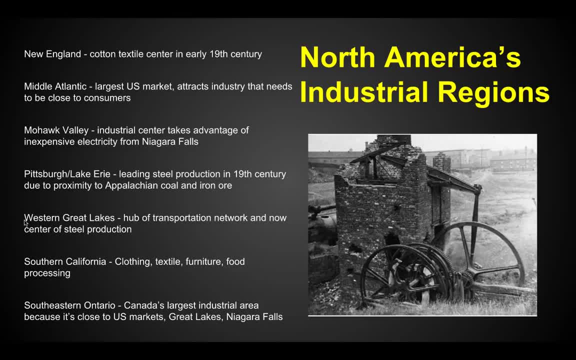 rolled into the processing plants over railroads in chicago. that's the western great lakes region, southern california- a lot of variable uh industry production there with closing- textile, house furniture, food processing, and southeastern ontario. it's canada's largest industrial area because it's close to the us markets. it has the great lakes and niagara falls for hydropower. 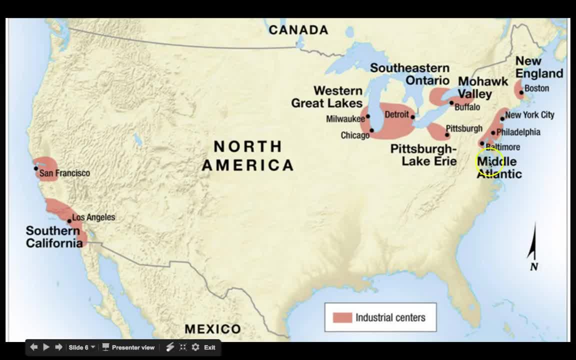 there's the graphic, so we're looking at the largest market here. of course we've got major cities like new york, philadelphia and baltimore. what you used to have is the center for steel in pittsburgh. here, proximity to coal in the appalachian mountains has now moved west to detroit.